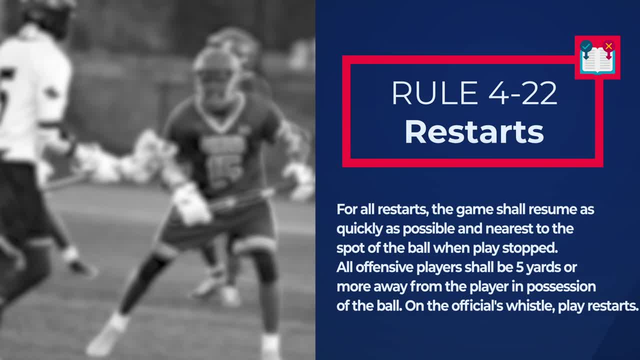 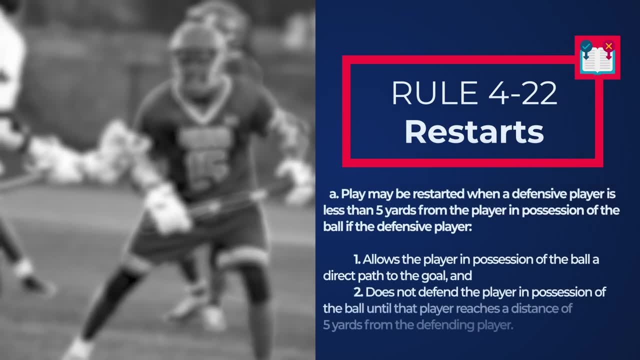 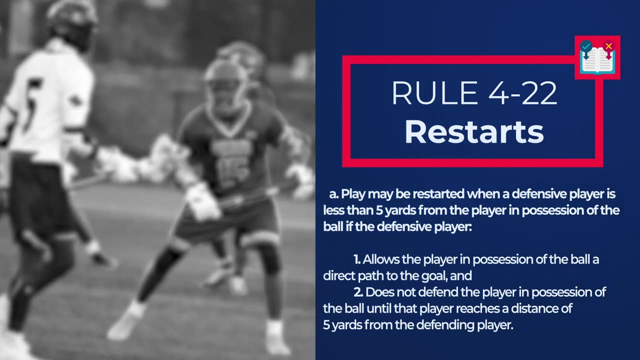 at or near where the ball was when play was suspended. Under the revised rule, play can restart when a defensive player is less than 5 yards from the offensive player in possession of the ball. If this situation occurs, the defensive player must allow the player in possession of the ball. 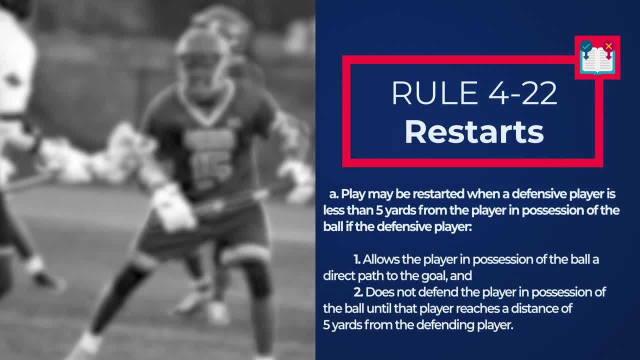 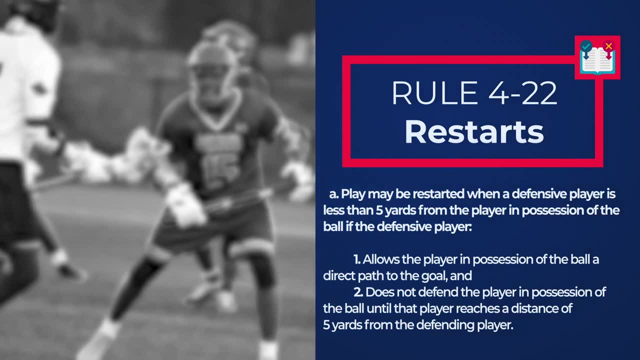 a direct path to the goal, and the defensive player may not defend or engage the player in possession of the ball until he has established a distance of five yards or more from the ball. carrier. Officials and coaches should make note in their 2020 rule books on page 51,. 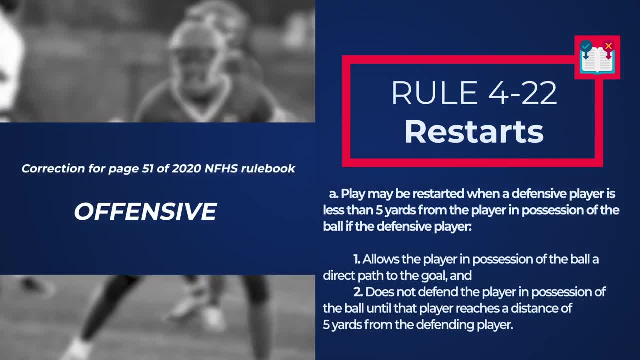 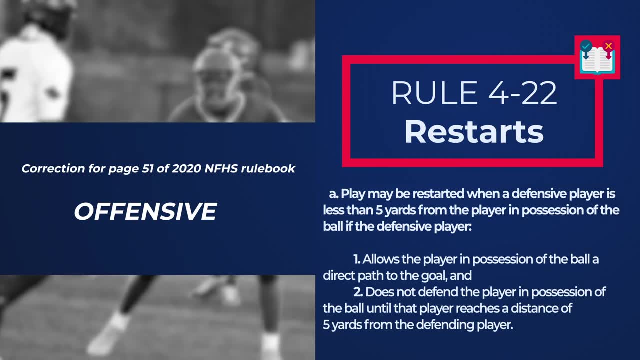 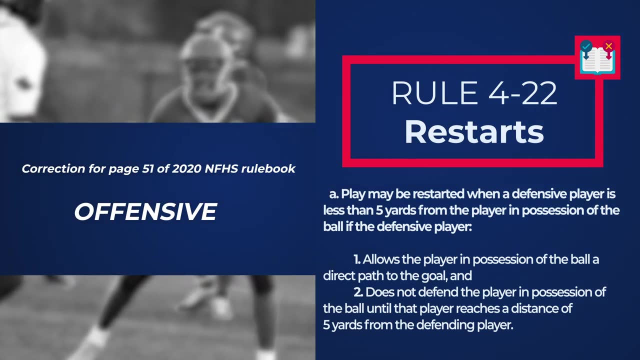 the word offensive was inserted to state all offensive players must be five or more yards away from the player in possession of the ball. This was done to clarify that only an offensive player can delay a restart Before play resumes. any defensive player five or more yards away from the ball carrier. 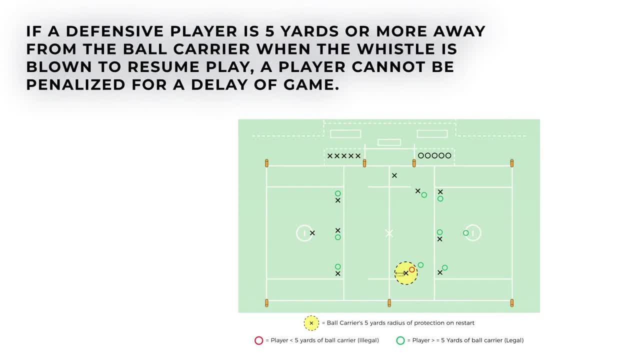 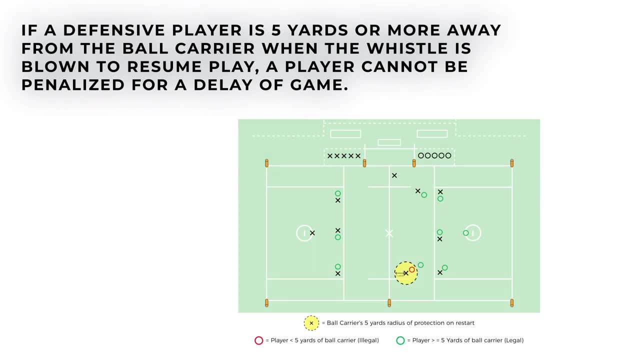 does not need to give the offense with the ball a direct path to the goal and are free to engage the ball carrier as soon as the whistle sounds. In the following example, you will see that one defensive player is less than five yards away from the ball carrier before play restarts. 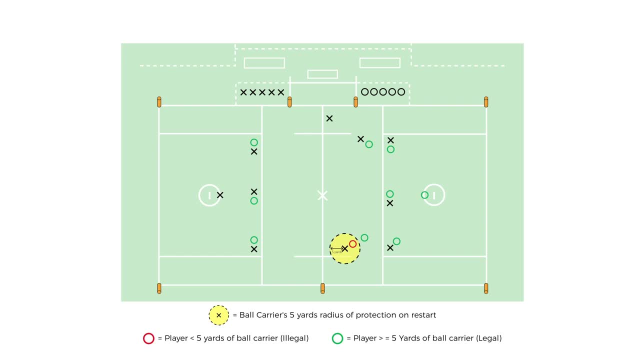 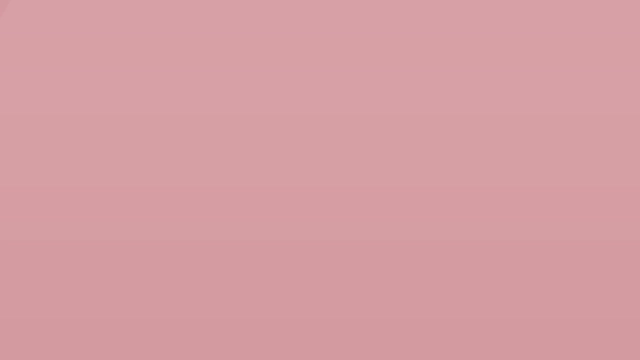 and all others are five or more yards away. Only the player less than five yards is required to give a direct path to the goal and can only defend against the ball carrier once he has gained a distance of five yards. If a defensive player is within five yards, 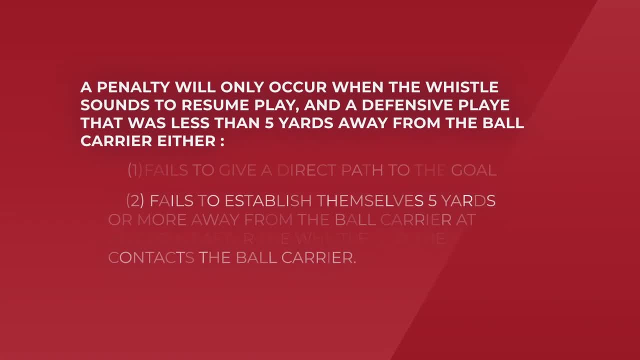 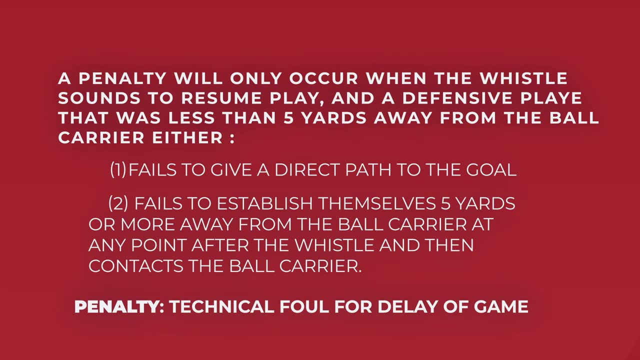 of the ball carrier. when play resumes, that defending player must give the ball carrier a direct path to the goal without impeding his play, and establishing themselves at least five yards away before playing defense on the ball carrier. Failing to do either of these will result. 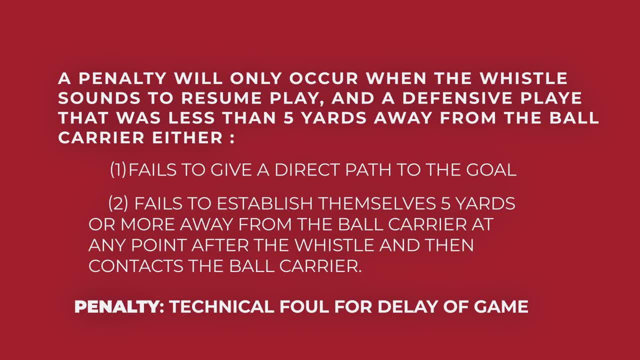 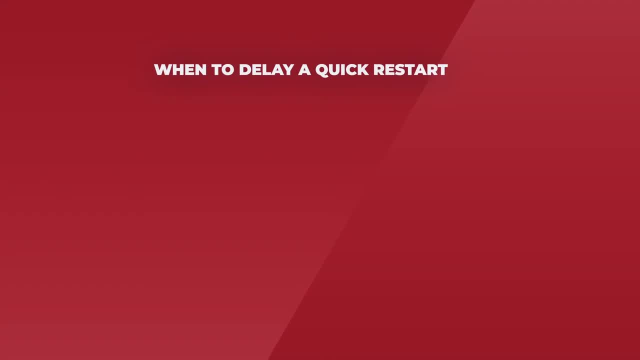 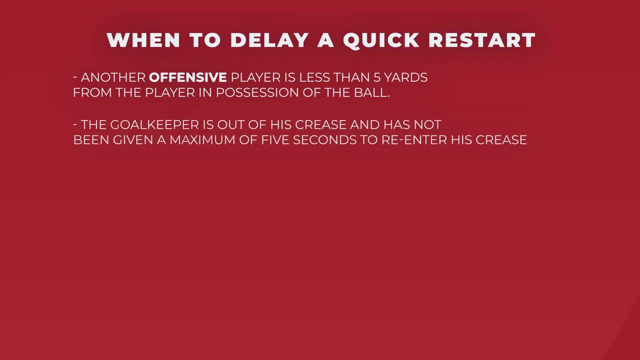 in a slow whistle situation followed by a technical foul for a delay of game. There are still instances to delay a restart. They include when an offensive player is less than five yards from the player in possession of the ball. When a goalkeeper is out of his crease. 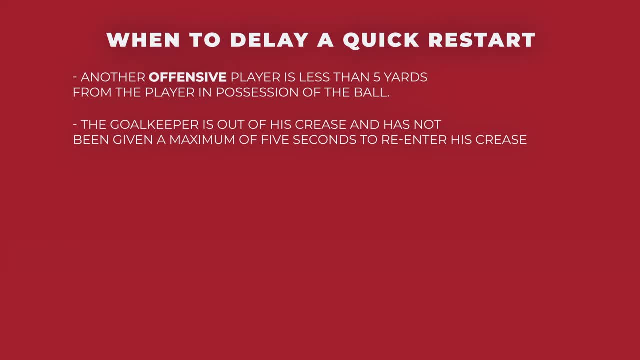 and has not been given a maximum of five seconds to reenter his crease. the ball carrier is required to give a direct path to the ball carrier on a restart When the player in possession of the ball is ready to restart play but is within five yards of the substitution area. 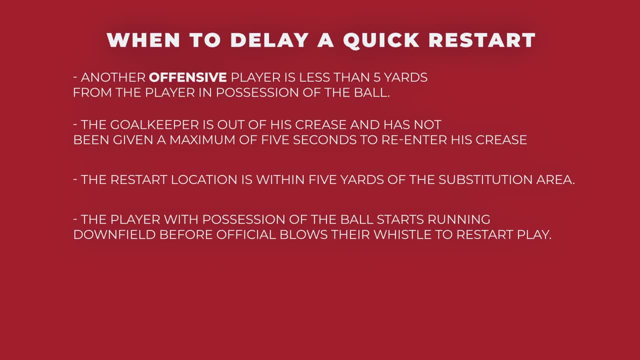 An unfair advantage gained by the player in possession of the ball starts running downfield before the official blows their whistle to restart play. When play is blown dead by officials and the ball continues to roll downfield away, a player will not be called out. 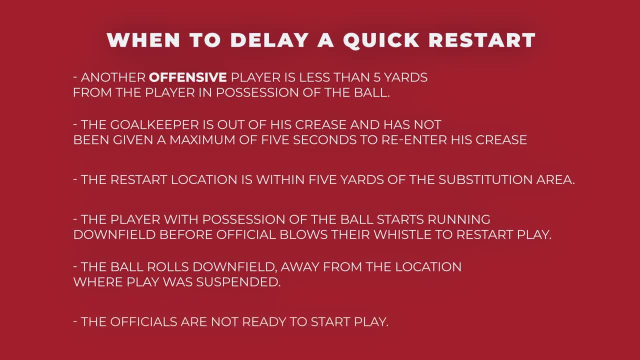 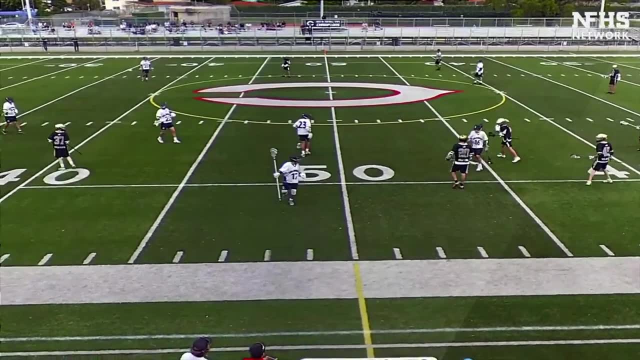 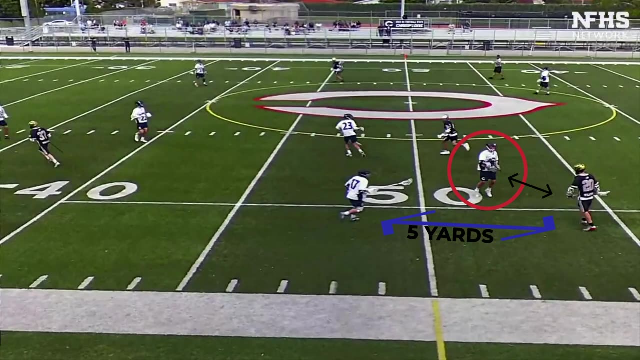 or an official is not ready to start play. In this first clip, after a loose ball violation, number 20- blue picks up the ball and plays restarted with number 16- white- less than five yards from the ball carrier. as play resumes, White number 16 immediately defends the ball carrier. 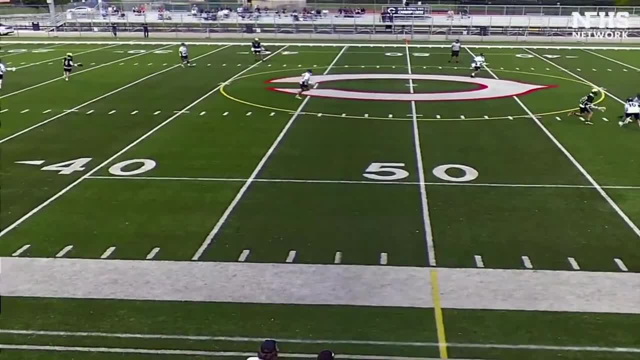 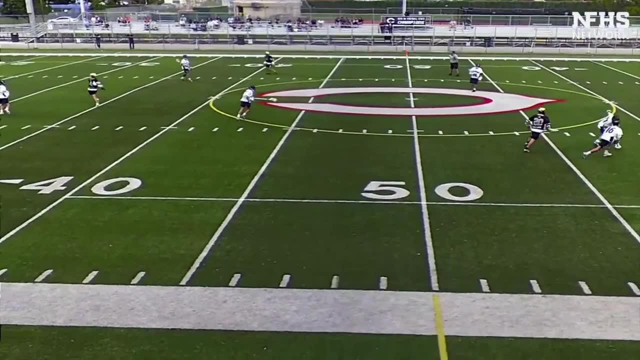 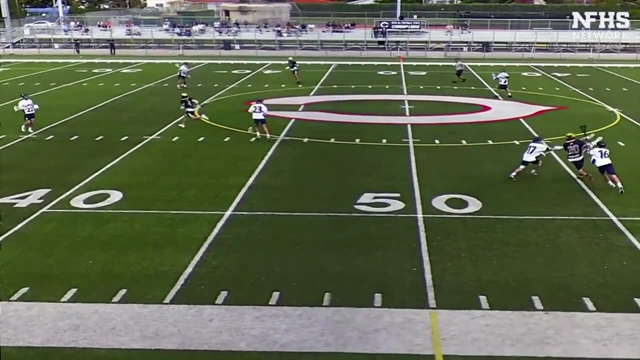 and is flied for a technical foul for delay of game because he did not establish himself at least five away from the ball carrier after the full ball, the ball carrier before or after the whistle and defends against the ball carrier. Pay attention to white number 17.. After the loose ball violation occurs, white number 17 did establish himself. 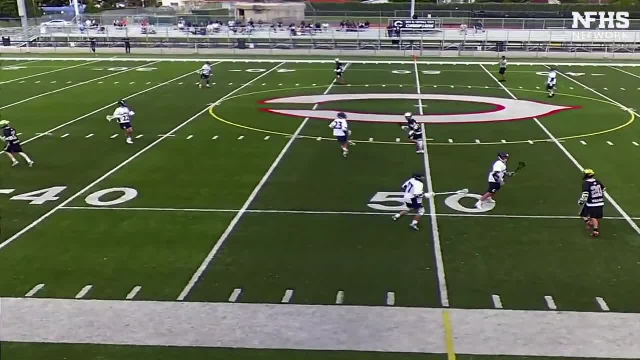 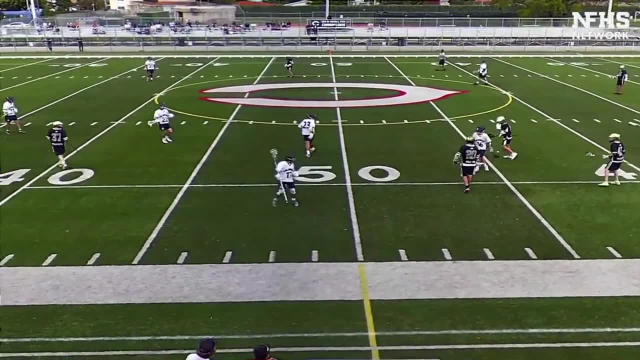 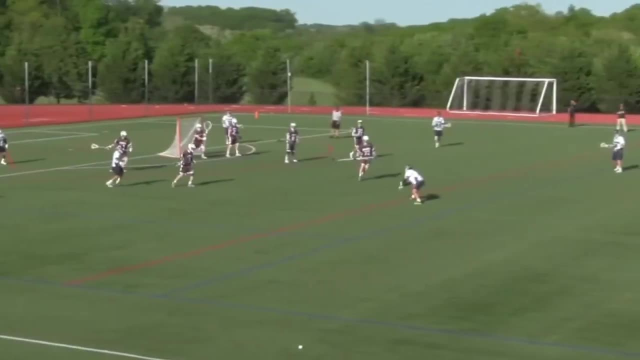 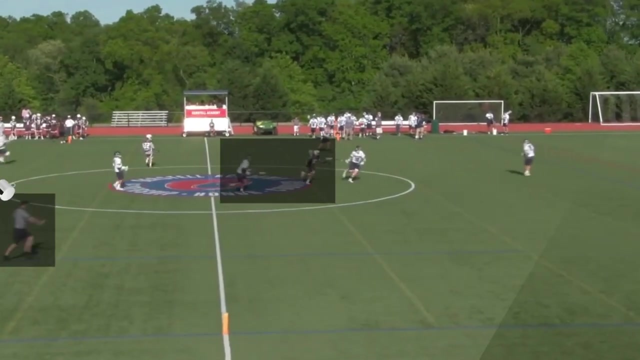 five or more yards away from the ball carrier. Because of this, he is free to defend against the ball carrier immediately. This next clip is another example of a defender not reaching a distance of five yards or more before defending the ball carrier After an over and back violation. 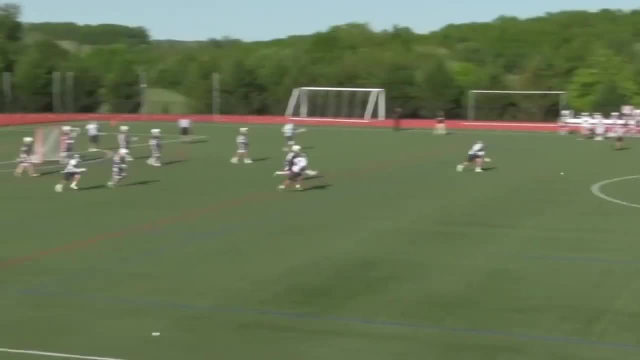 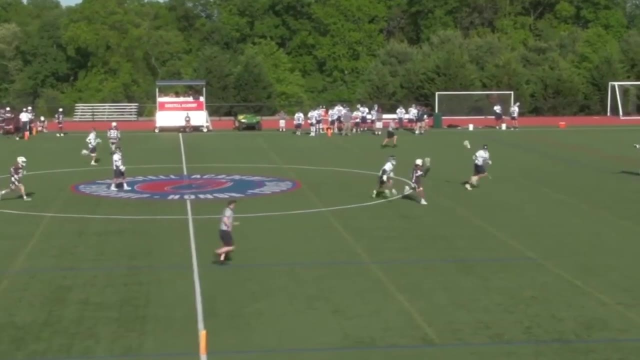 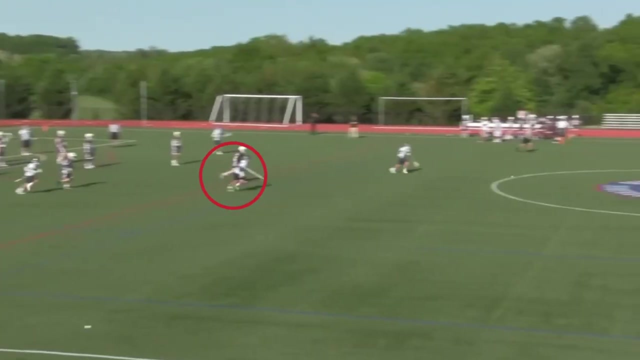 attack man number 12 on the brown team picks up the ball and play is resumed quickly by the officials. Number 13 white is at a distance which is less than five yards from the number 12 brown when the official blows the whistle to resume play. Because number 13 white? 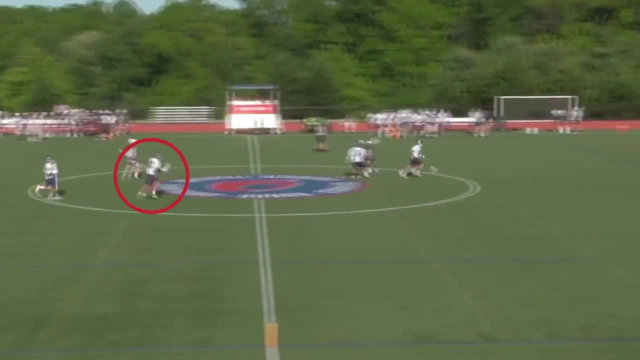 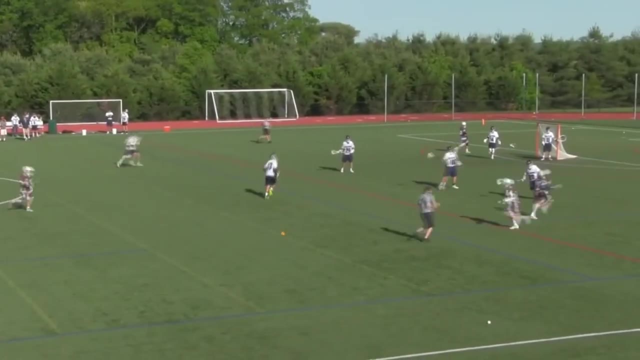 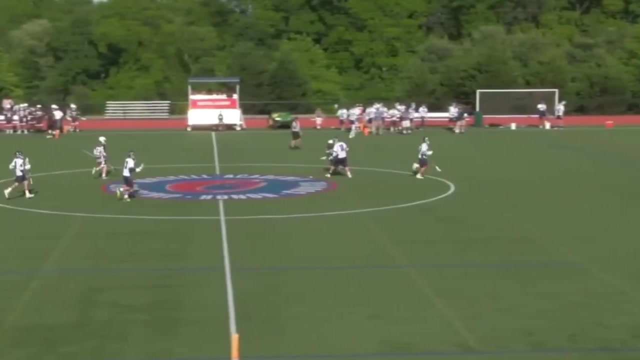 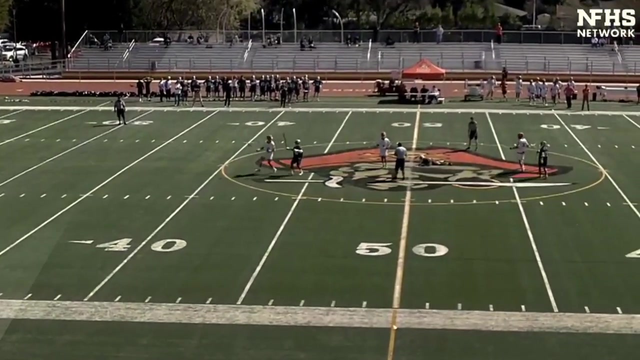 contacts the ball carrier and never established a distance of five yards or more, the official throws the flag on number 13 white for a technical foul Delay of game. The following clip is an example of when a second offensive player is less than five yards from the. 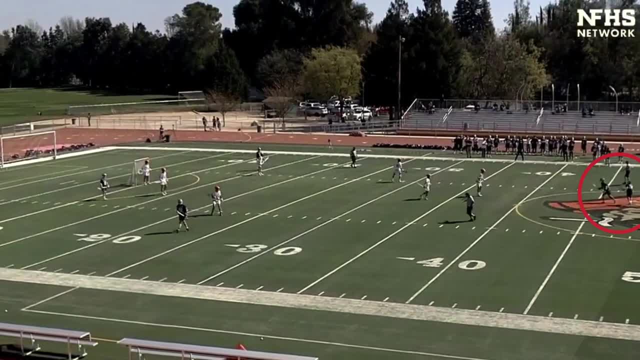 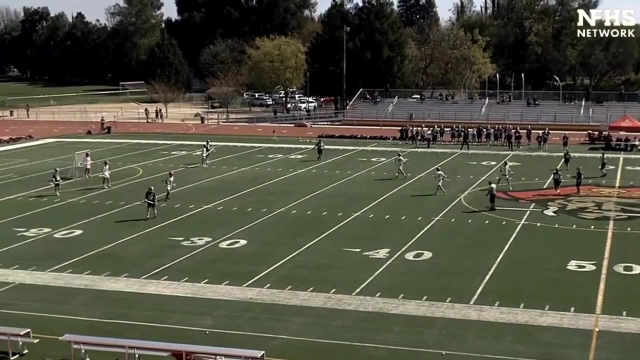 ball carrier when played. It is still a requirement that all offensive players be five yards or more away from their teammate before play can resume. If this situation occurs and officials inadvertently restart play, they should stop the game immediately, return the ball carrier to the correct starting location and properly restart the play. 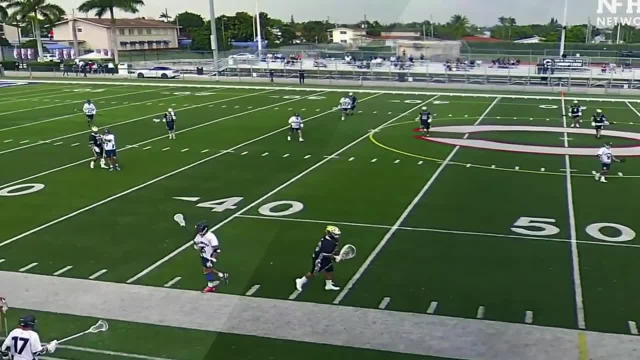 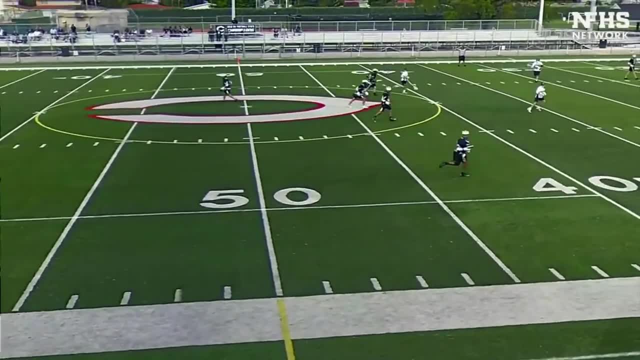 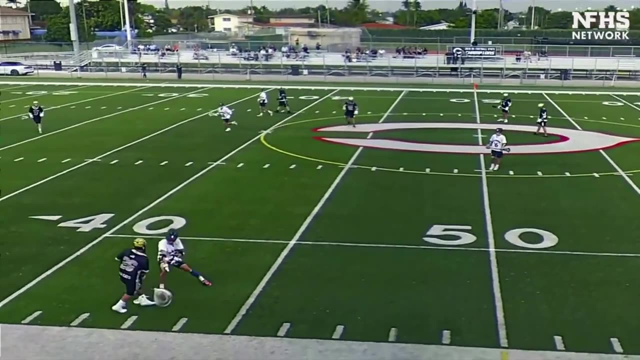 This next clip demonstrates a goalkeeper who is not able to play National Olympian of Ohio. Richard Suarezzymnick and cayonna doesn't look good as their team. sorry, the punter for painkillers. it's good they get balls located in the Deadline appendix. 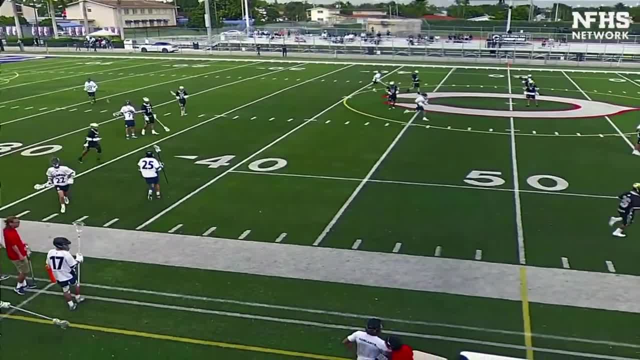 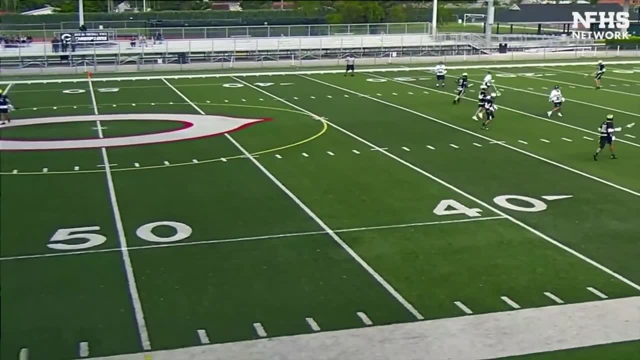 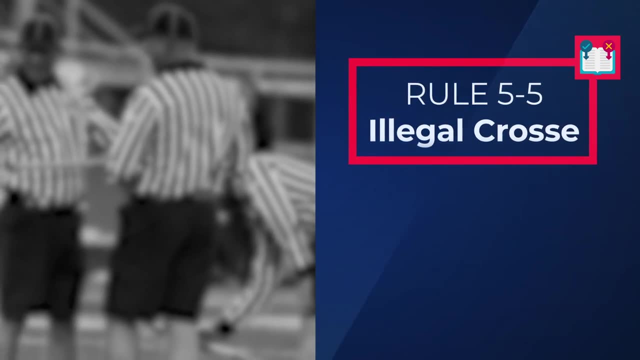 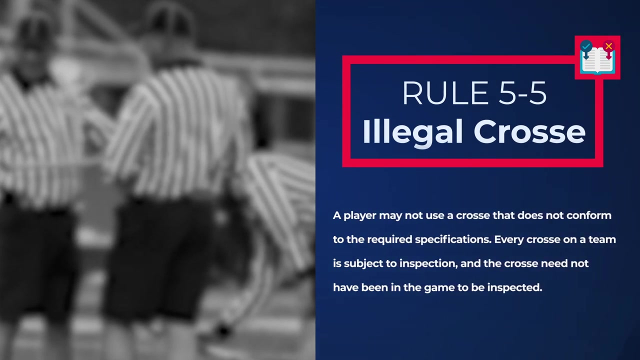 is bтак Mara War Burgos V VerdN I. Napoli preside a defeat. He played just 55 per game in baseball. five illegal cross: all crosses that are found to be illegal when inspected by an official during a game carry a personal foul penalty time of two minutes. non-releasable illegal cross penalties. 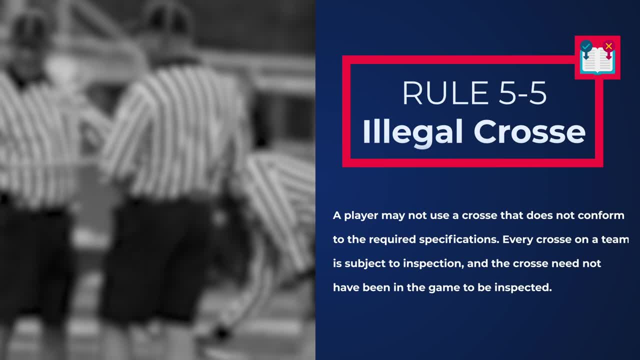 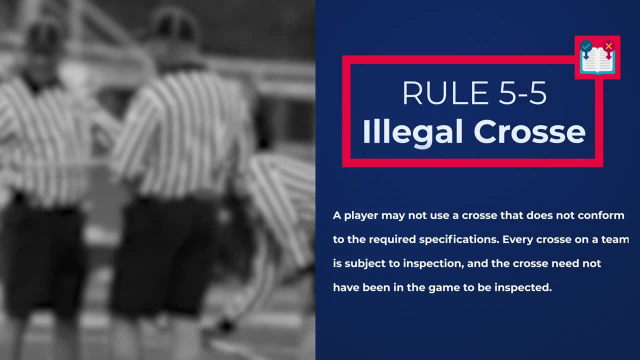 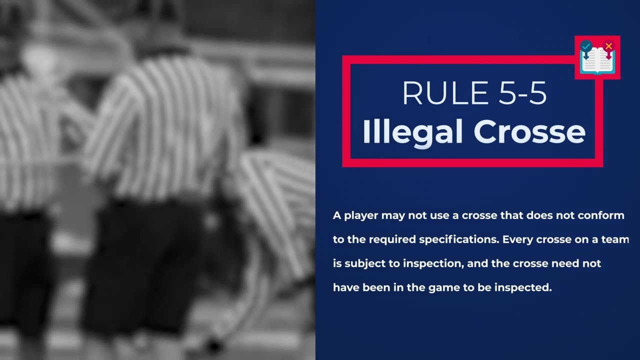 are no longer of the one minute or three minute variety. the two minute foul replaces the previous illegal cross penalty times, in which some issues were correctable and carried a penalty length of one minute and other cross penalties had a penalty length of three minutes and the player's cross remained at the table for the rest of the game. it is the responsibility of the player. 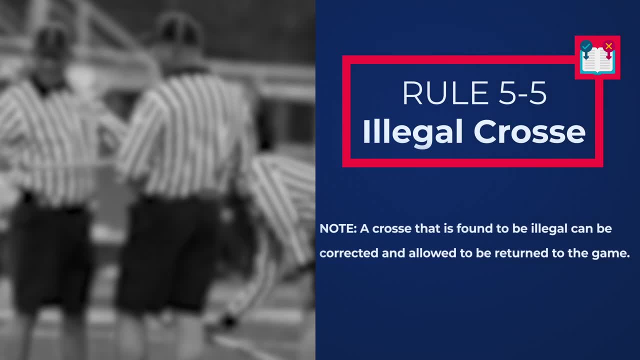 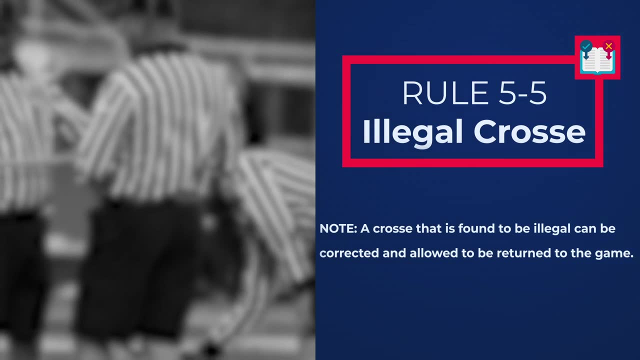 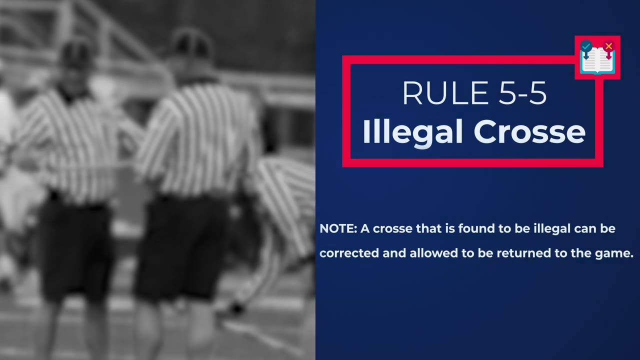 and coach to assure that the stick is legal for play. if it is used again in a game, the officials do not re-inspect a cross to ensure it is legal for play. if a cross that was already found to be illegal is found to be illegal again later in the game, it will result in a new two-minute. 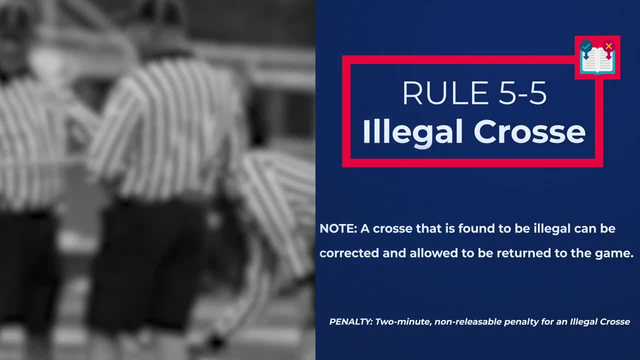 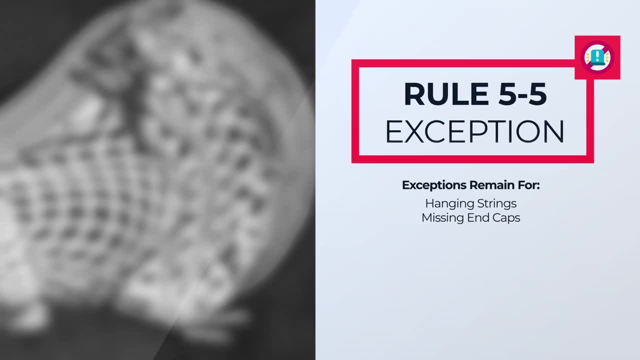 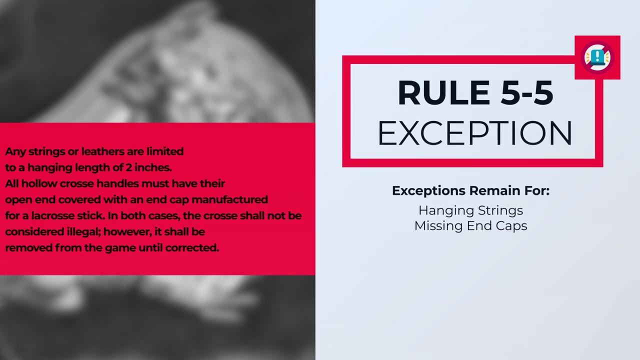 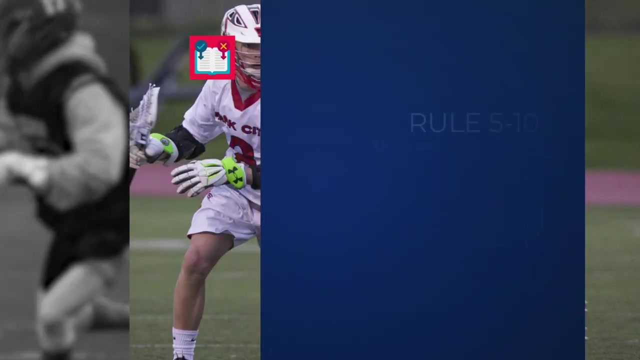 non-releasable personal foul for any legal cross. exceptions remain in the rules for hanging strings or a missing end cap. both of these issues, when identified by officials, can be corrected without penalty, provided the player fixes the problem before returning the cross to the game. rule 510: unsportsmanlike conduct: throwing a cross at the ball. 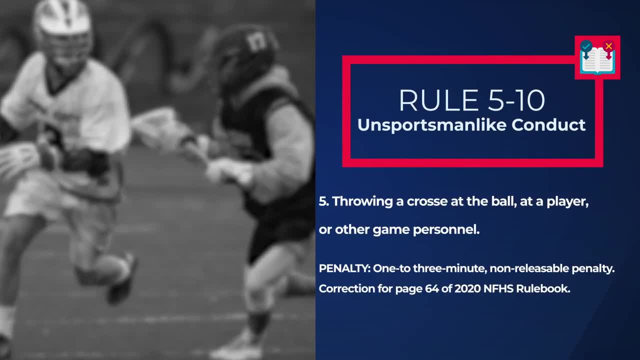 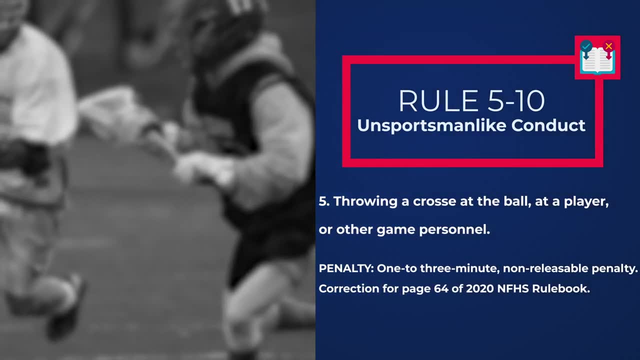 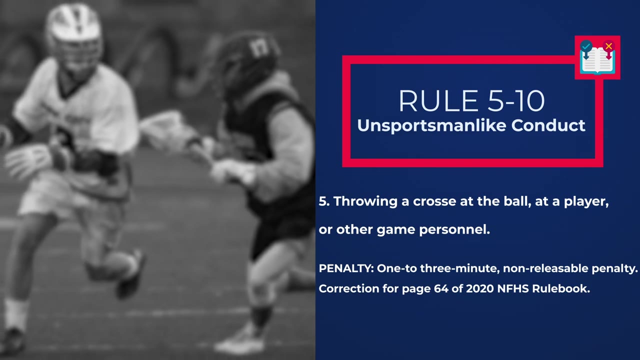 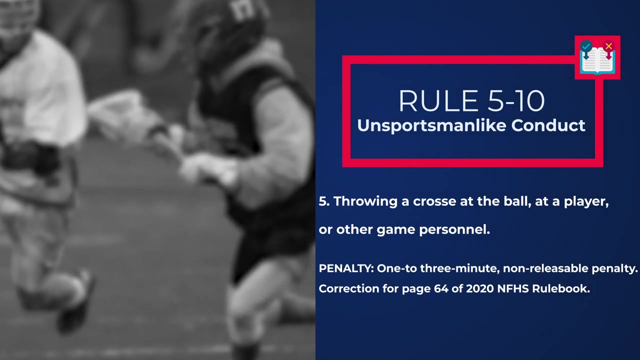 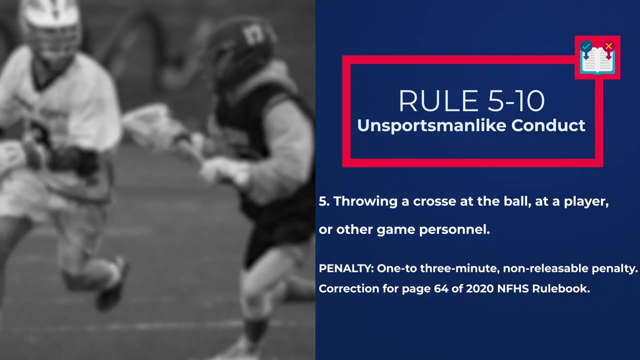 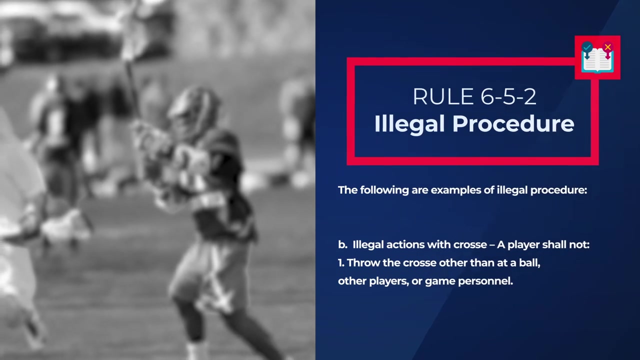 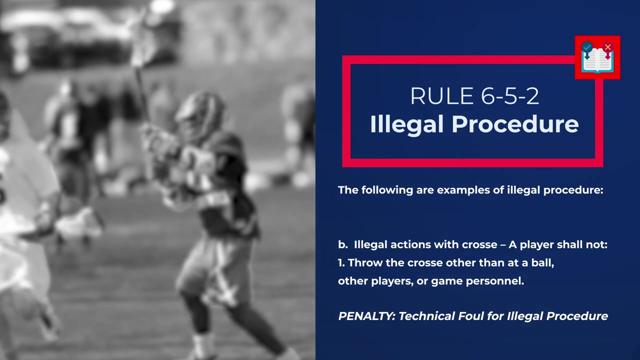 another player or other game personnel is penalized as one to three minutes. non-releasable penalties- rule 652: illegal procedure. throwing the cross for any other reason other than what is listed as an unsportsmanlike penalty is penalized as a technical foul for illegal procedure. 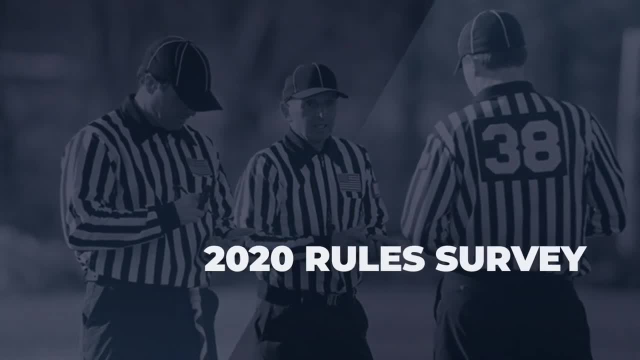 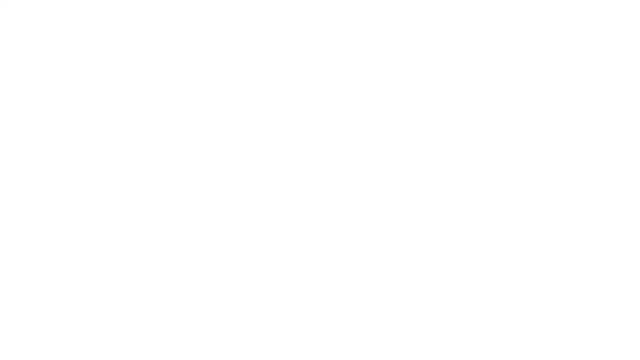 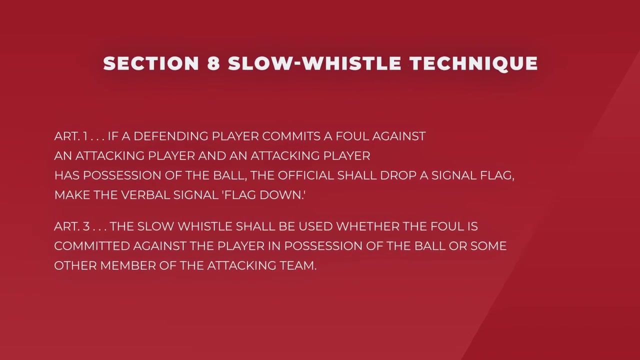 the 2020 nfhs rule survey results indicated that coaches and officials continue to be confused on slow whistle situations. the slow whistle technique allows a play to continue temporarily, so the offended team has an opportunity to score a goal after the defending team has committed a time serving foul. 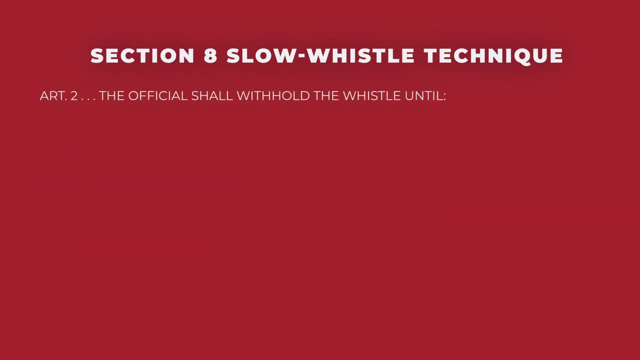 the slow whistle stops when either a goal is scored, the ball goes out of bounds, the defense gains possession of the ball, the offense commits a foul, officials stop play for an injury, or a player that lost a piece of equipment that causes the foul, or that person lost an…. 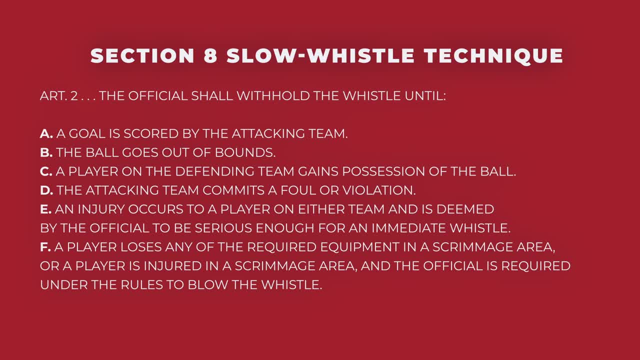 therefore that player will face theOLTRA designed penalty andlement penalty to raise the score. though. all defensive mira helmet contain a negative penalty. if the defense loses the, that causes a potential safety issue. a timeout is called the end of a period. a second defensive 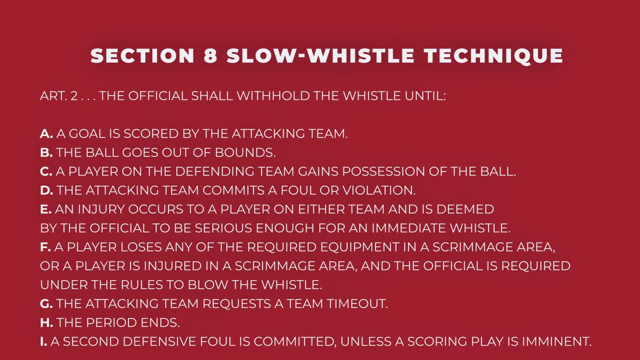 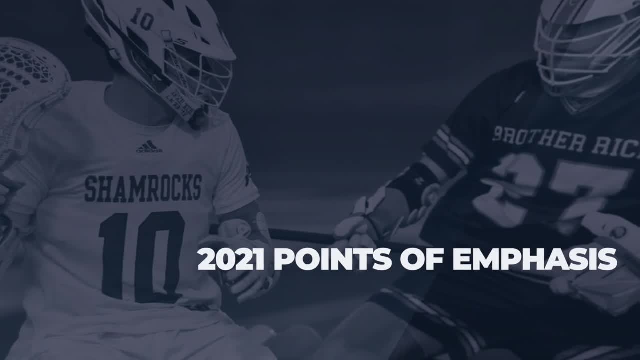 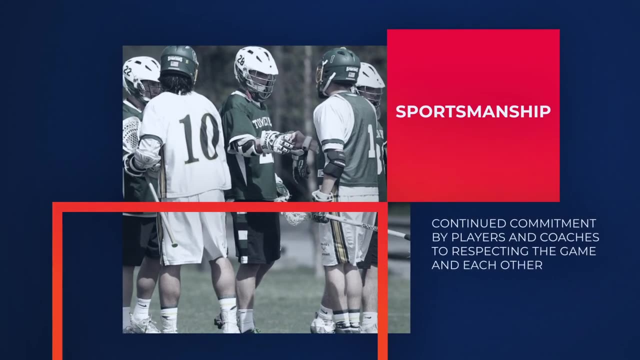 foul is committed. The NFHS Boys Lacrosse Committee would like the lacrosse community to be aware of the following points of emphasis for the 2021 season: The NFHS Boys Lacrosse Rules Committee advocates for the continued commitment by players and coaches to respecting the game and each other. 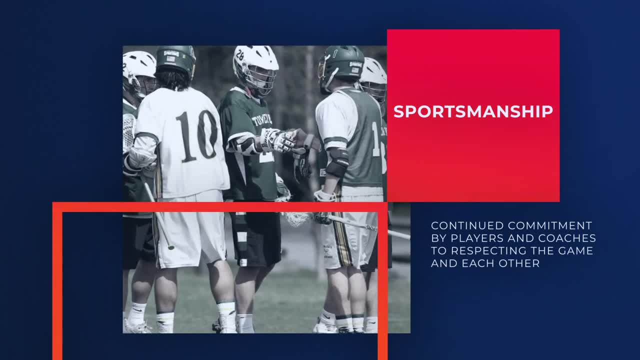 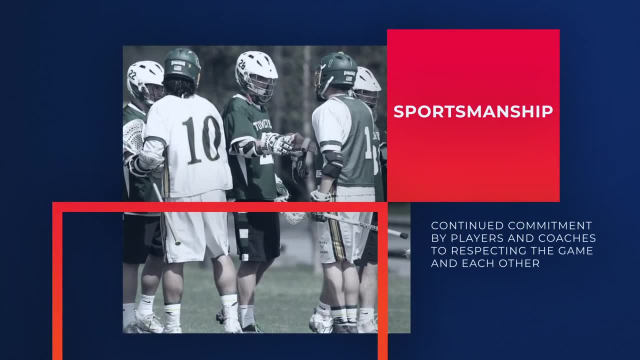 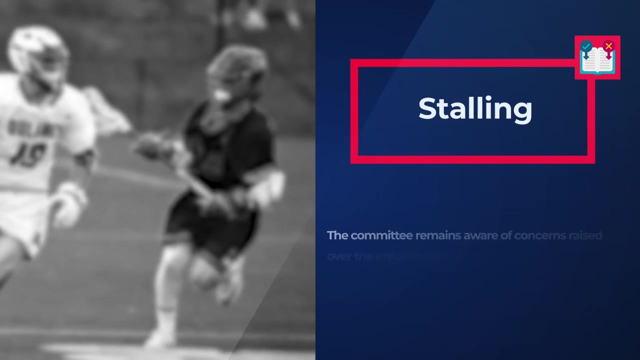 Head coaches should monitor and discuss sportsmanship with their players and assistant coaches to ensure the game is held to the highest standards. The Committee expects all participants to continue to work together to exhibit good sportsmanship from pre-game through post-game. The Committee remains aware of the concerns raised. 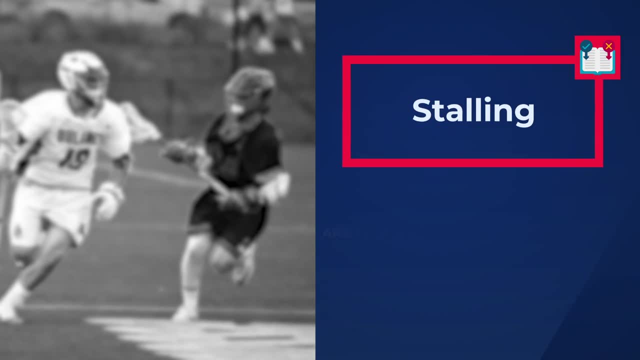 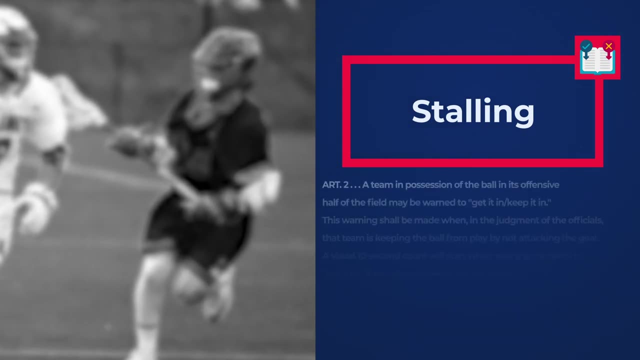 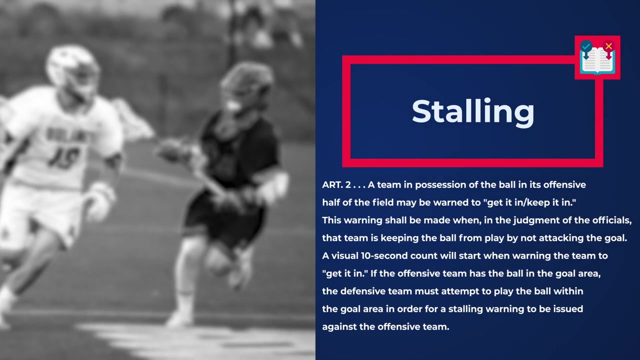 over the last year and a half, It is the responsibility of the team in possession of the ball to attack the goal. Stalling rules can only be enforced once a team has successfully cleared the ball into their offensive area and appear to be, or are deliberately not, attacking the goal. 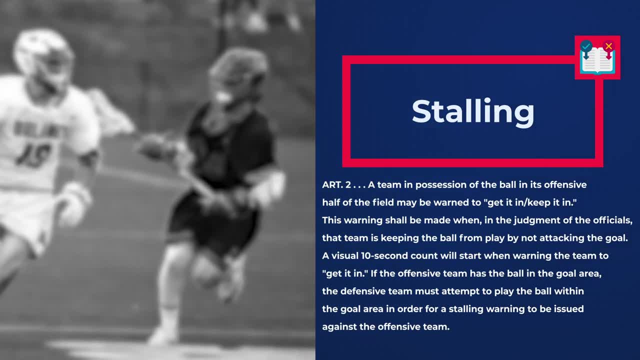 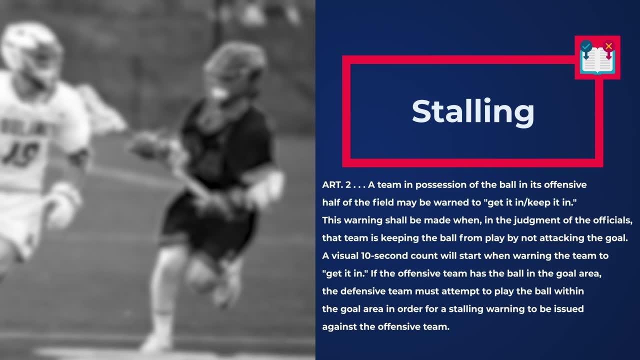 As a reminder, stalling can be enforced whether a team is man up, man down, winning or losing in a game. Stalling cannot be called if a team has possession of the ball. A stall warning can be issued, not shoulders above the Indian hand near a block and or. 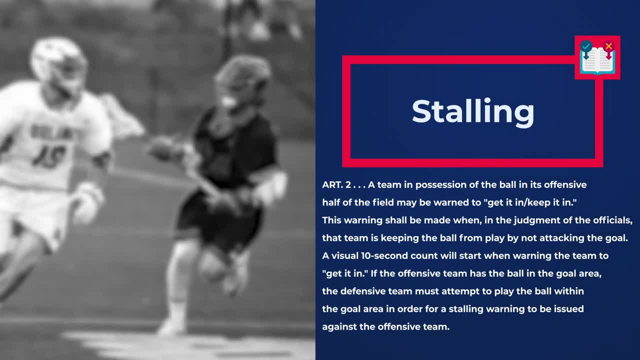 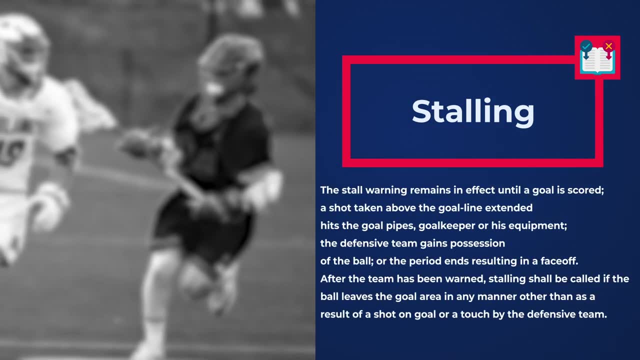 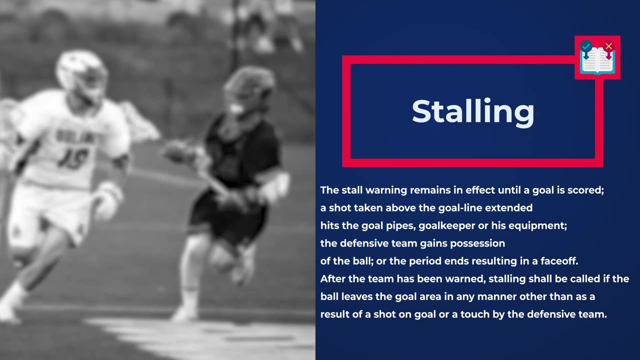 outside of the group's line-up. Then when the ball arrives in possession of the ball- a signesin swamping the goal. A stall warning remains in effect until a goal is scored, A shot is taken at or above the goal line extended that hits the goal. pipe's goalkeeper. 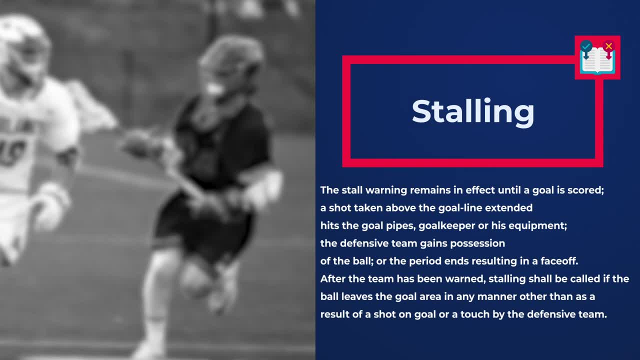 or his equipment. The defensive team gains possession of the ball. The period ends resulting in a face-off. The goalkeeper listens intently until prove Dakler hit the true contact with the pipe. Be prepared, lateERROLFcom, to see a troutisesti when it plays the four lights on the field. 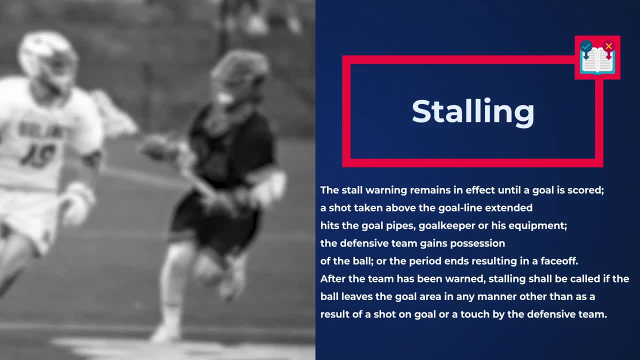 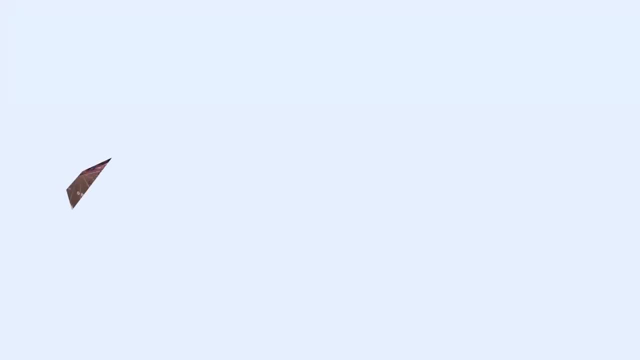 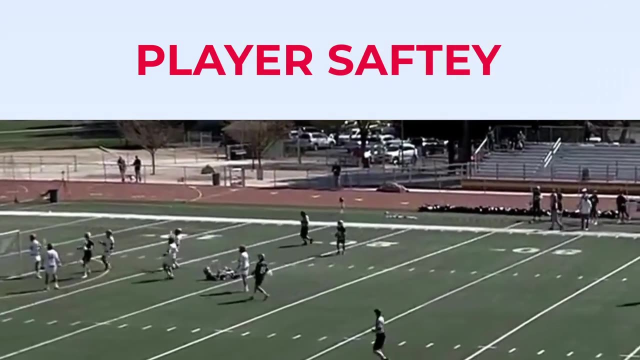 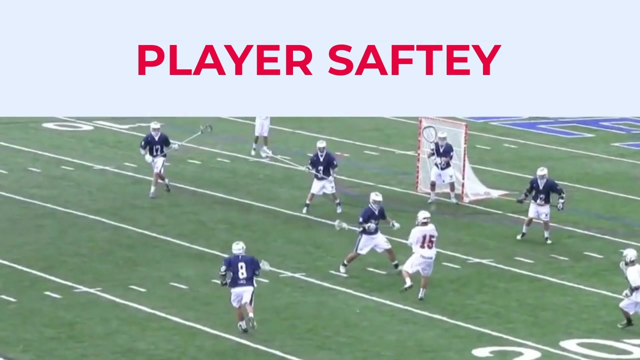 The committee encourages coaches and officials to review the rules and situations that apply to stalling before the start of the season. Continuing emphasis is needed regarding player safety rules. specifically, illegal body checks, checks to the head or neck area and targeting Contact to the head or neck shall result in a two or three minute non-releasable penalty. 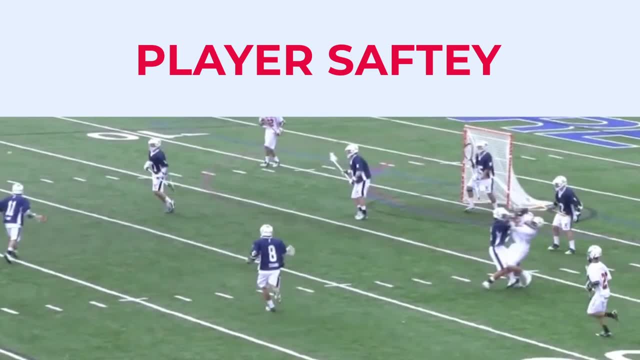 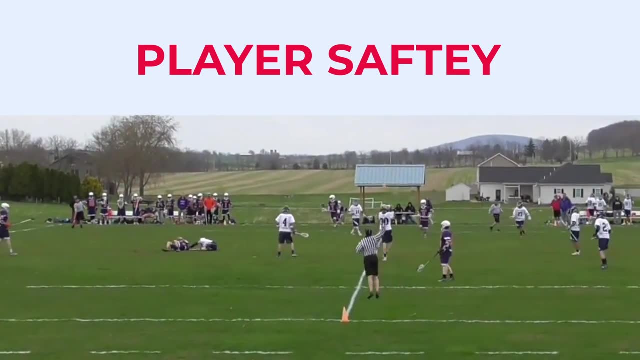 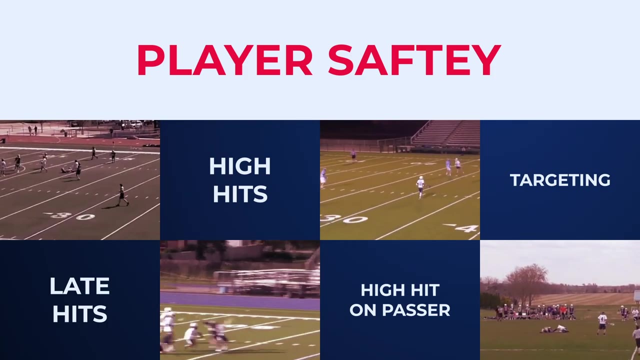 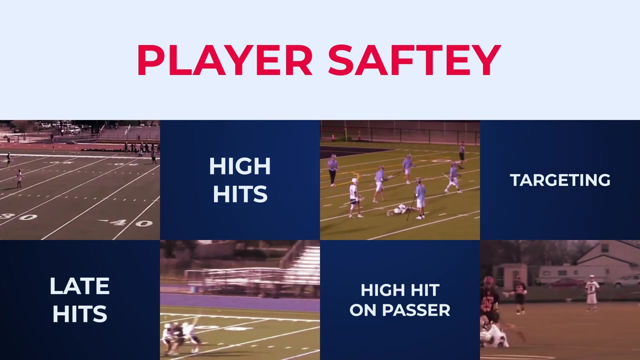 A two or three minute penalty occurs whether the initial contact is made directly to the opponent's head or neck or a legal body check slides up into the opponent's head or neck. Players shall not body check a player in a defenseless position. Hitting a defenseless player also will result in a two to three minute non-releasable penalty with the potential for an ejection.